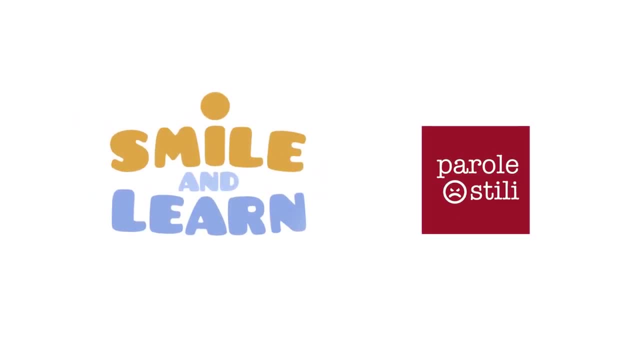 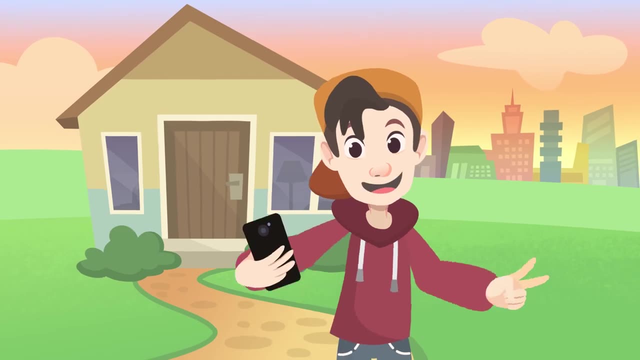 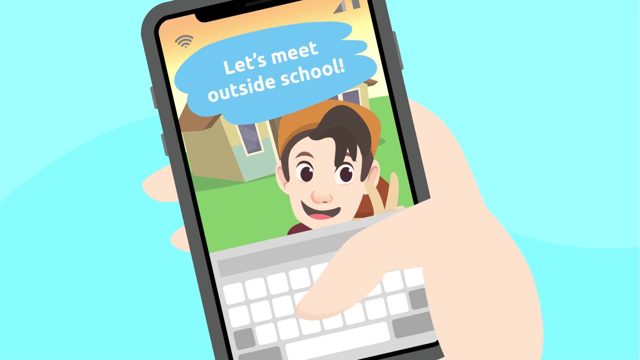 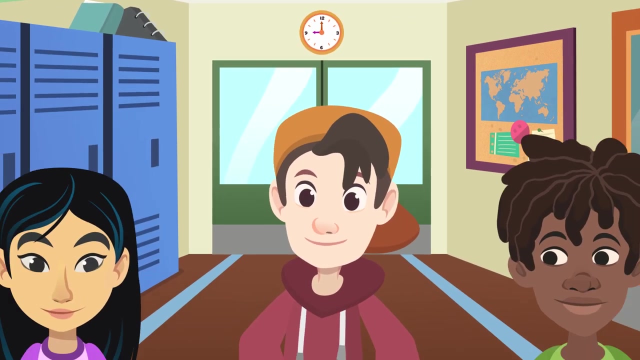 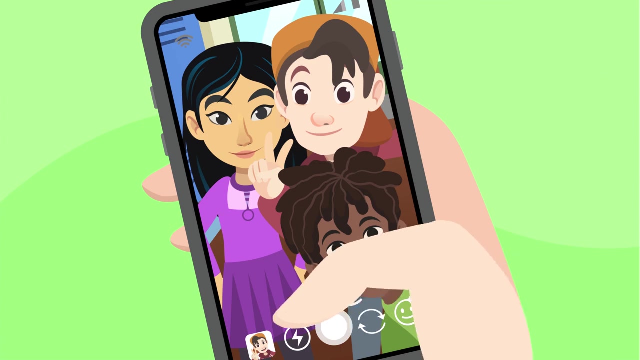 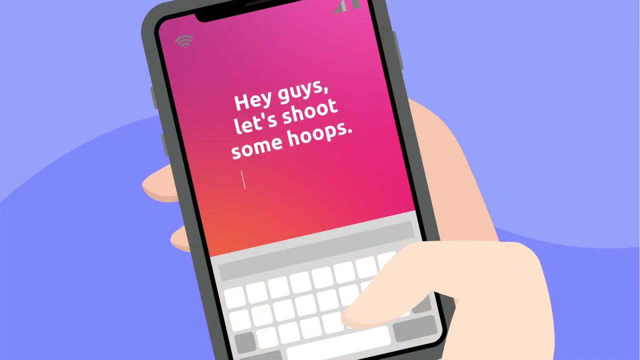 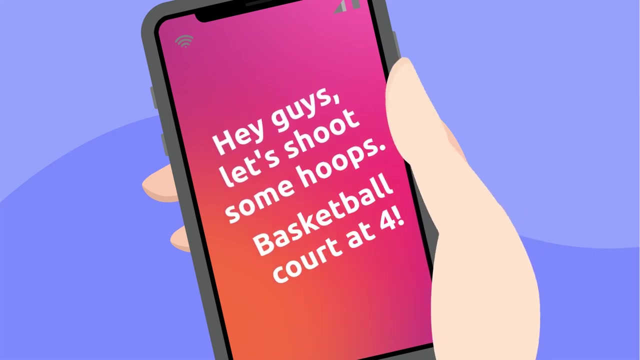 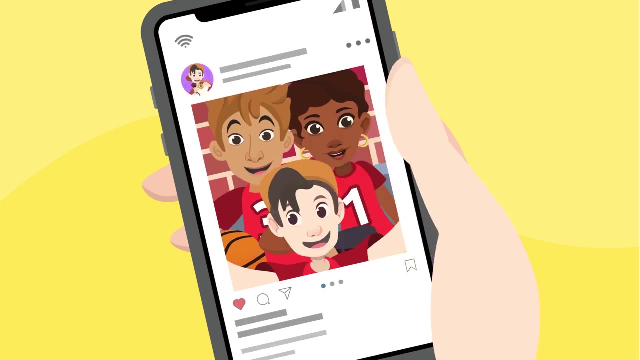 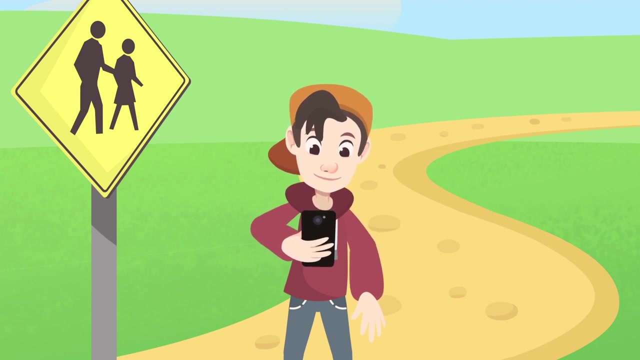 Today is my birthday. I'm going to post a story. Let's meet outside school. Happy birthday Selfie. Yeah, Hey guys, let's shoot some hoops: Basketball court at 4.. I'll be waiting for you at my place to celebrate. This is my address. 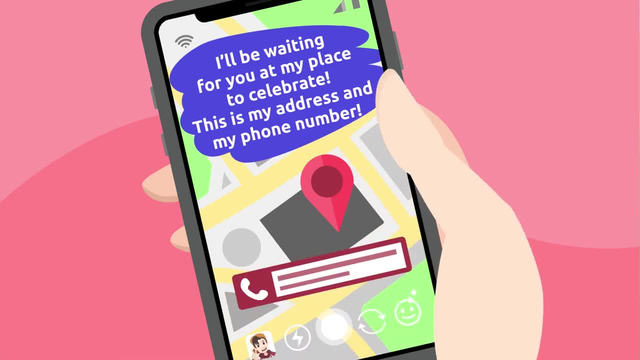 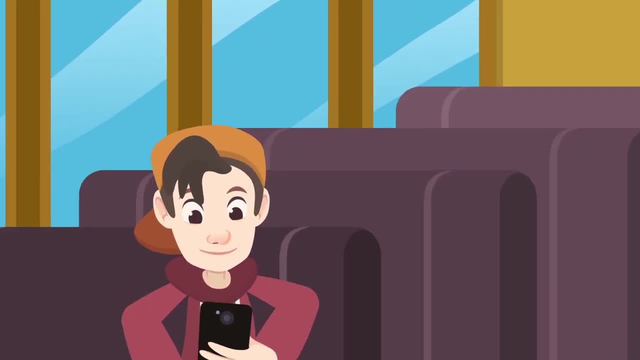 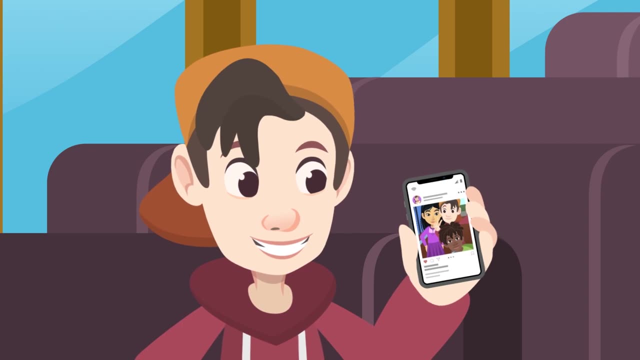 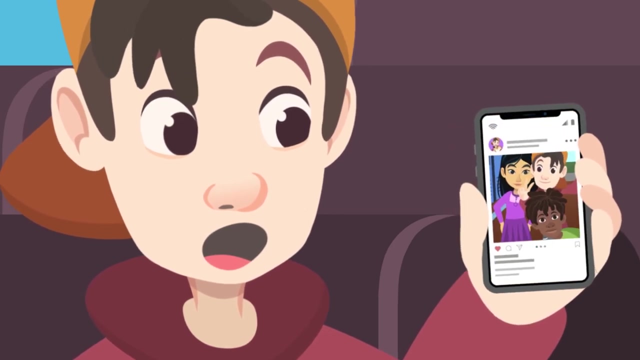 And my phone number. Happy birthday, David. You're very popular, aren't you? You have lots of friends. You use chats and social media all the time. They know everything about you. What you like when your birthday is who your friends are, the sport you play. 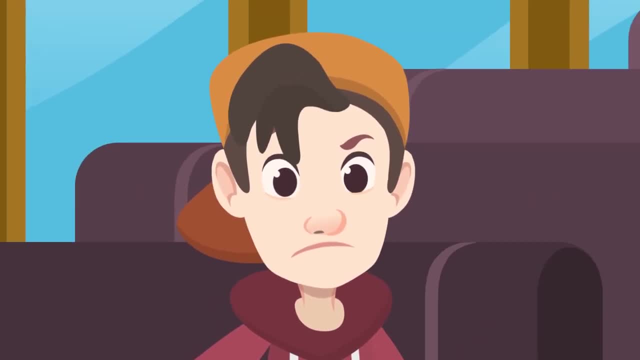 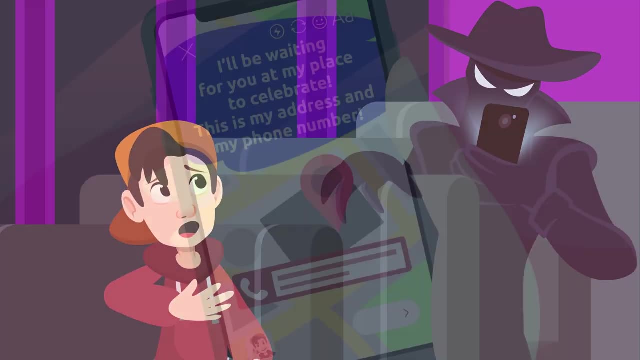 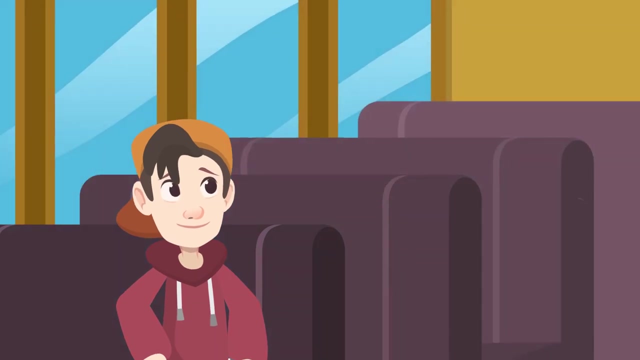 But they could also know your phone number and where you live. Have you ever thought that what you share online could be read by someone that is not so much of a friend? Always remember to take great care with the personal information and photos that you share online. 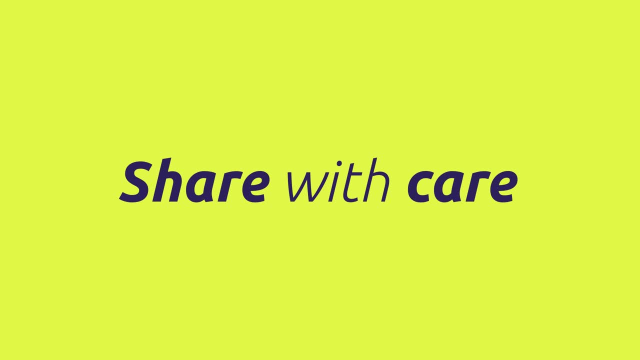 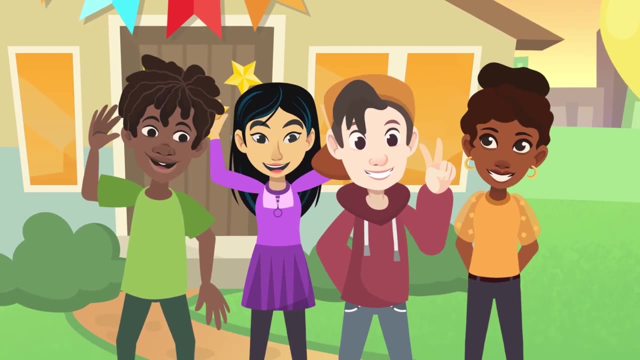 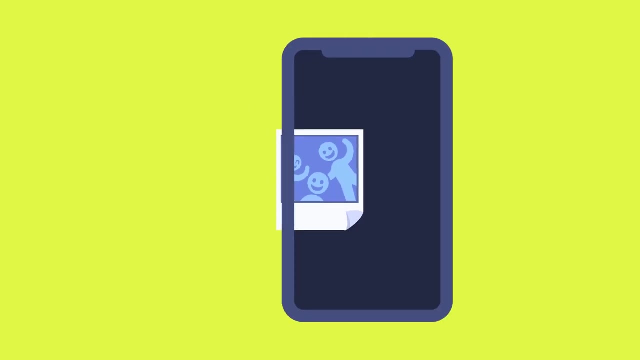 Share with care. Now let's go celebrate. Your friends are waiting for you. Tentatively. no one can come to see you until you put colors on your 목 Bundesliga. Remember: Pictures and information that you post or send can be easily re-shared by others. 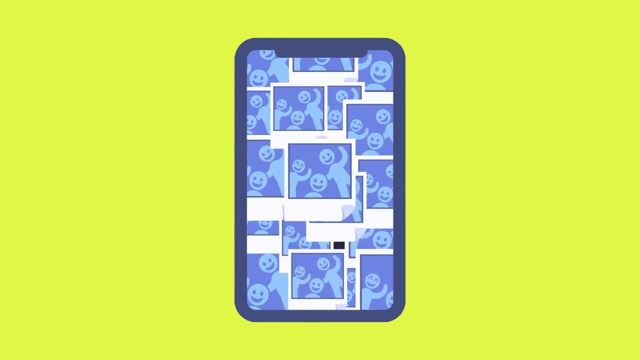 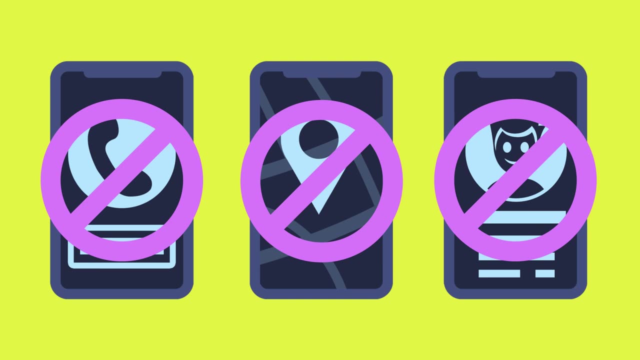 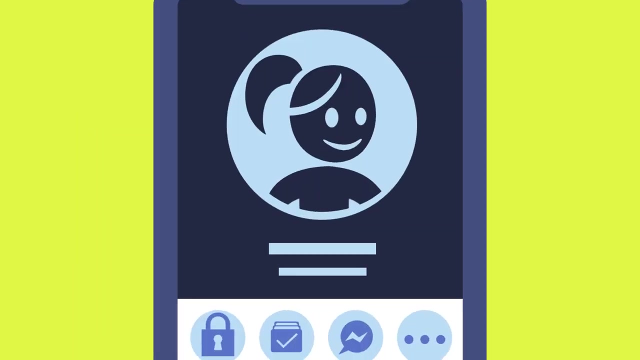 so they could remain online for a very long time. Be careful when posting. Don't share phone numbers, addresses or personal details. This information could be misused by others. Don't post photos and information on Facebook, Tinder and social media. Always check your privacy settings of the apps you use. 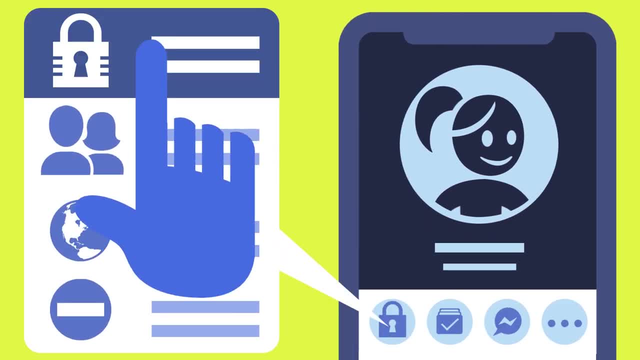 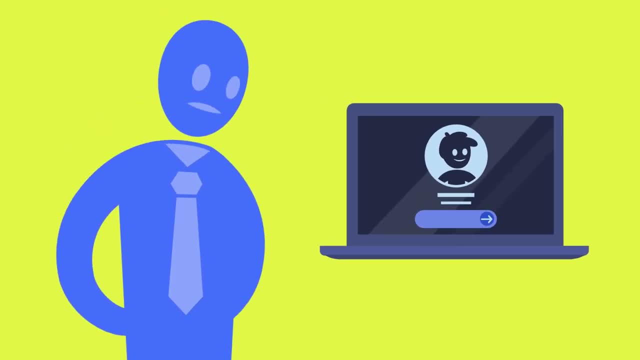 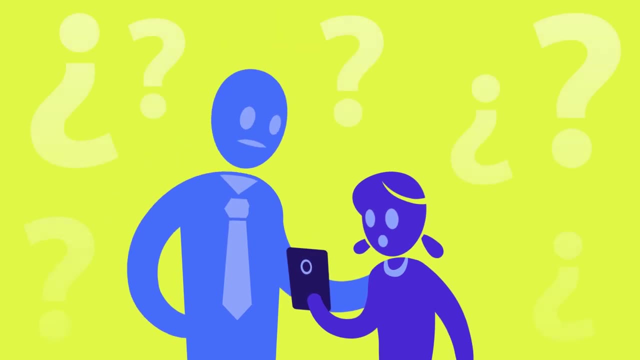 It's important to know what people can see or who can contact you When signing into a website or social media. ask an adult for help and advice. Choose a difficult password and share it only with your parents. Take great care with everything you share online.